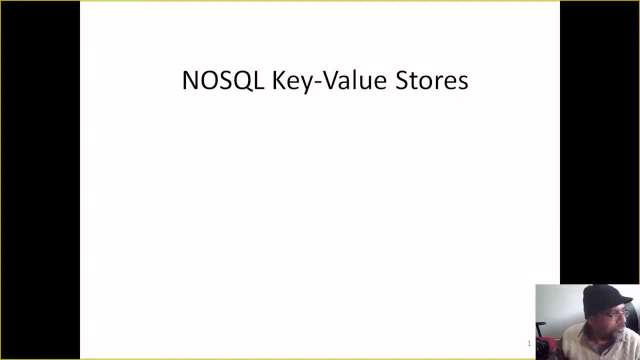 more and more So you will see here, and many problems can be easily modeled using this key value data store And the development of this key value data store can be easily done with the help of SQL database. The key value data store was because of the SQL database was not able to capture or able. 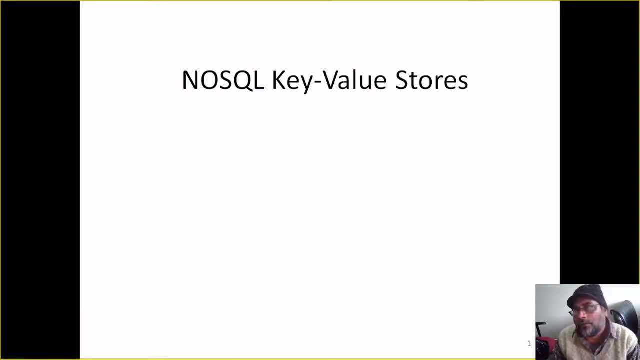 to model the requirements of the new e-commerce or web-based applications And this key value database came into existence. And, based on this principle, today many key value databases can be used. Many key value database are available, Few are open source and others are proprietary. 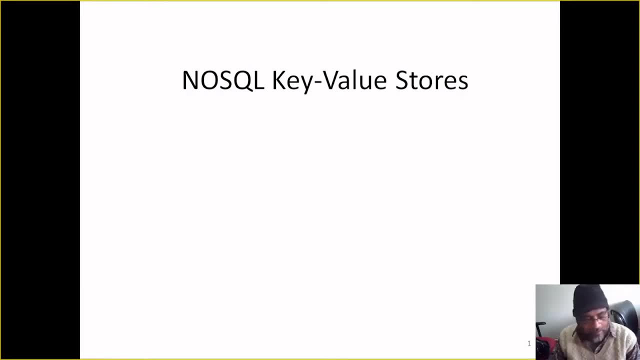 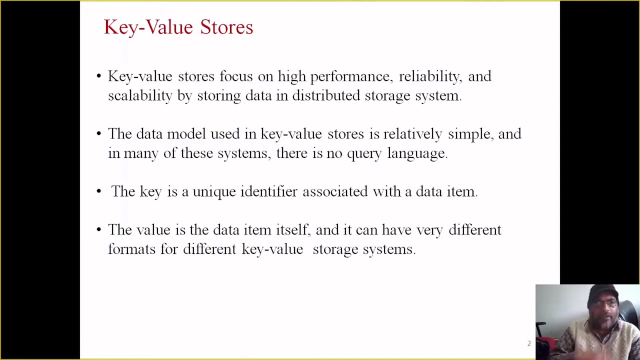 product also. So today we will see what is this key value data store and what are the examples of key value data store And some more thing that is consistent, consistent, consistent, consistent, that I will show you. Key value store or key value database, same thing. So key value store, key value stores. 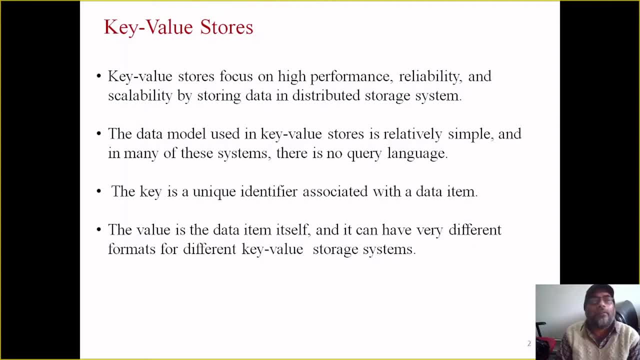 focus on high performance, reliability and scalability by storing data and distributed data. The data model used in key value stores is relatively simple And in many of these systems there is no query language. This is very big advantage that user need not to learn any. 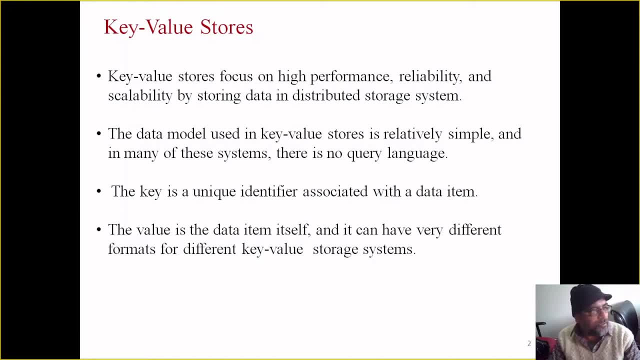 query language for using this SQL database. The key is unique identifier associated with a data item, As in the relational database. you know SQL database. The key is unique identifier associated with a data item, As in the relational database. you know SQL database. And the key is unique identifier associated with a data item, As: 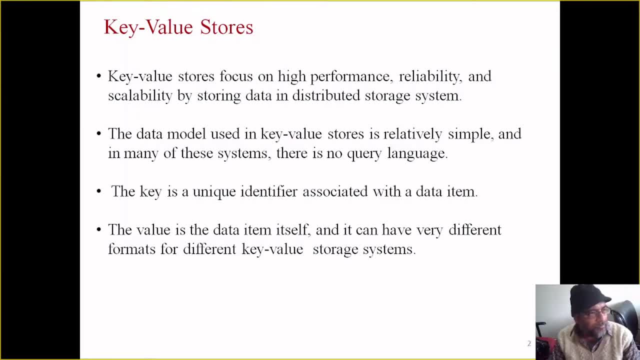 in the relational database, you know SQL database And in many of these systems, you know SQL database. These types of data store or key value data store are considered unique, the state, actual guidance, and then there is no query, perceptive and turn of each other. 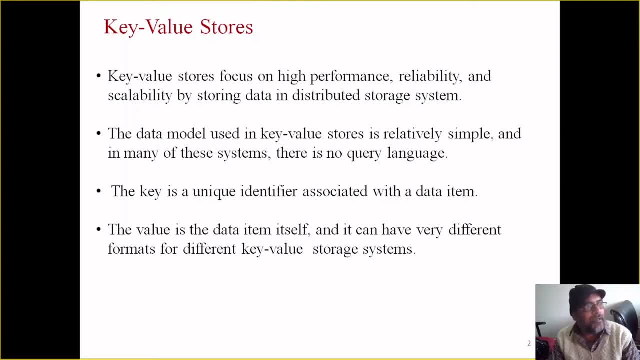 So here one more part that we can see and i'll show. we can also write in YoYo private identifier five column list. So, as you can see, there are a lot of written information here. We can think what is about a data item and what is about a�חנו article form. 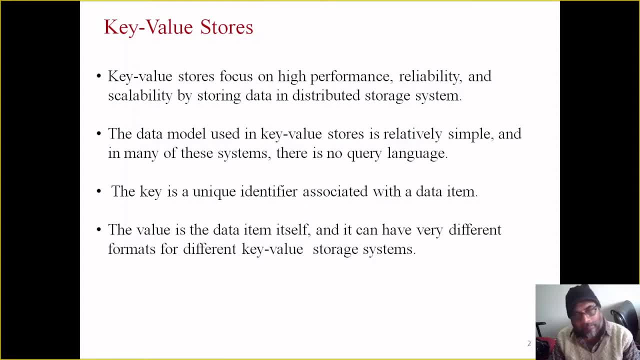 I will tell you how. data item value or simple value- and that can be of any type, any form. it can be a small value and it can be very complex data item also. so key is a unique identifier associated with a data item. the value is the data item itself and it. 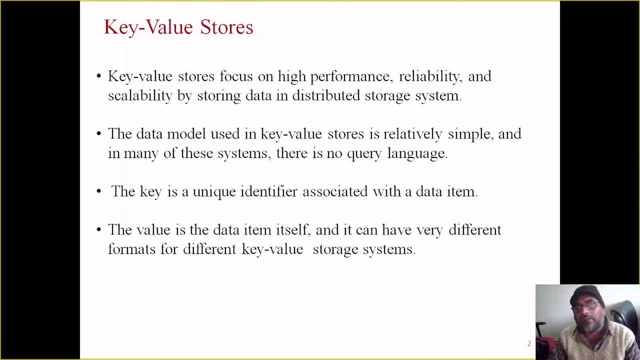 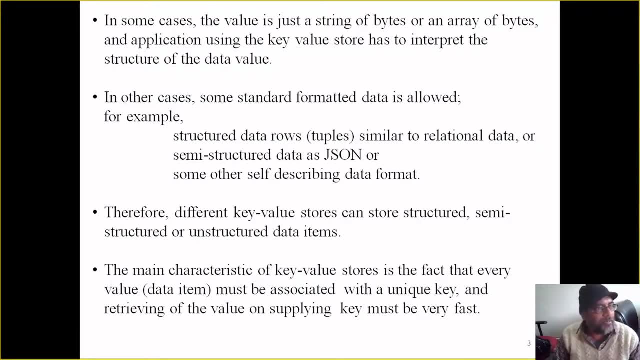 can have very different formats for different key value storage system. when we say the value can be of any kind of format, ok. so somebody say generally in programming we have integer type, we have we have other number type. we have several other kind of string type. we have string number type. we have string number type. we have several other kind of string type. 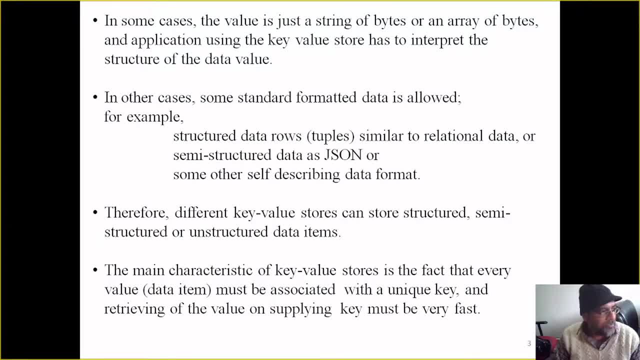 and other number type. we have several other kind of string type in the chamber type. we can see at that 있죠 app and we have certain everything type. we can see this layer with the services cables flow on at the sesame table And somebody can say real number, floating point, short, integer, long, integer, so many kind of types. or somebody can say they are different formats of the values. They are supported by the programming languages. 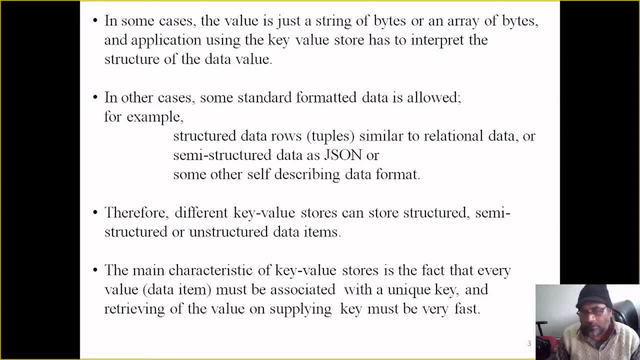 But here you see, in this database it says that it is simple byte. But what is this byte being represented and to what this byte has the representation? So it is responsibility of the programmer or application program To what it want to define. So, based on the program, the byte can be treated as integer, it can be treated as one document. also it can be treated as one record. so many things can be possible here. 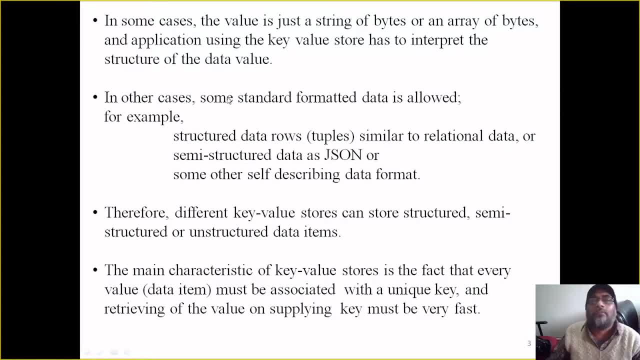 So in other cases some standard formatted data is allowed, For example structured data, wrote data Similar to relational data, So value can be triple, entire, complete triple. also It can be semi-structured data like JSON record And some other self-describing data format. 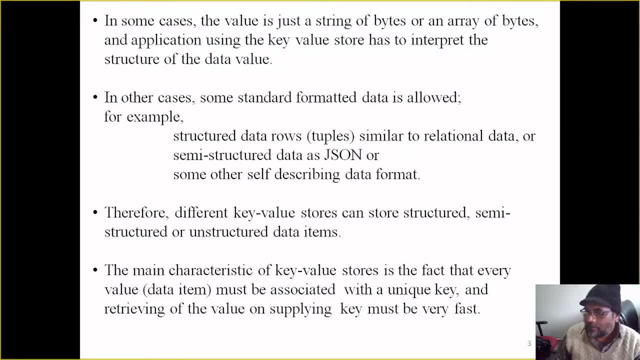 The application will define its meaning and it will interpret it. So therefore different key value stores can be used And can store structured, semi-structured and unstructured data items. So here any kind of data item can be represented or can be used with this key value store. 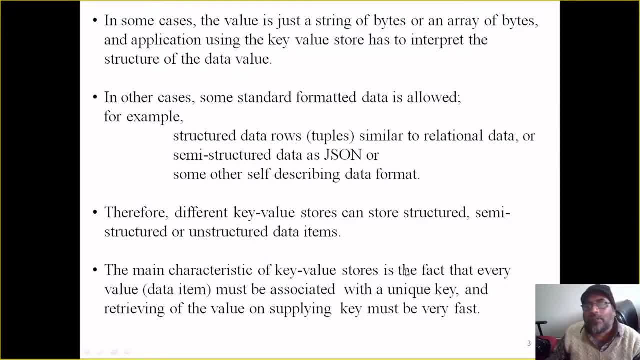 The main characteristic of key value stores is the fact that every data, every value data item must be associated with unique key And retrieving the value on supplying key must be very fast. Here, objective is only the key. will be associated, only one specific value. 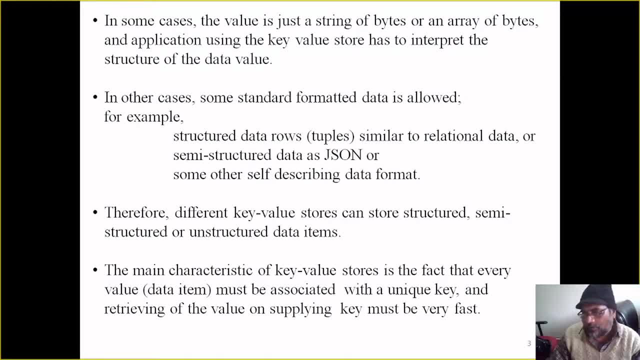 That is key value association. Other things are not defined, So that's why retrieval of data from the database will be fast. So many other processing that generally the relational database used to do is not present here. So one objective: first retrieval and second, association with unique key value of the data item. 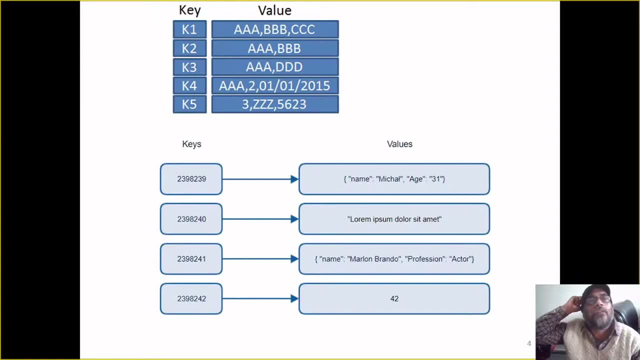 You can see this. You can see this is examples of key value. Suppose this is key, It has different value: k1, k2, k3.. And they are different values. This is one complete a this value. It has only two value. 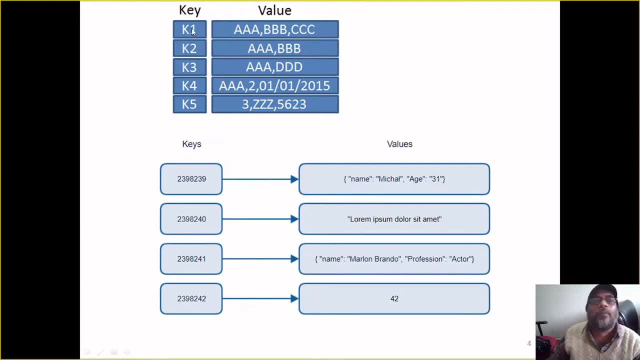 This is one again So different value. But when we say k1, that means this: a, b, b, b, c, g, c. This complete value is represented Similarly, and here you see key, Here some the other numeric values. 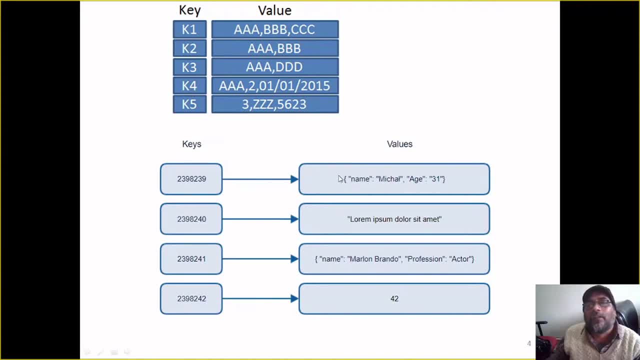 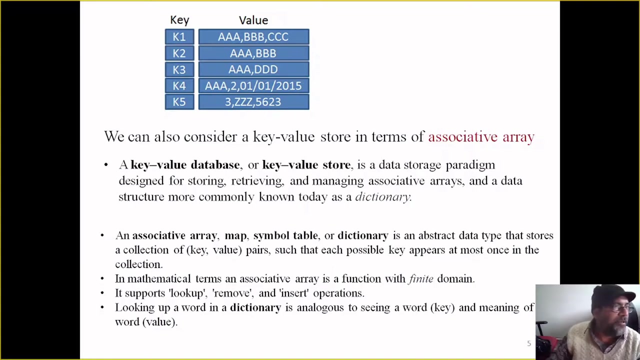 And this is representing this entire. Okay, This is So here only simple 42 number And it can also have this. So value can be of any type. Okay, Type is not being defined here. Type definition: it will be interpreted by the programmer for the application program. 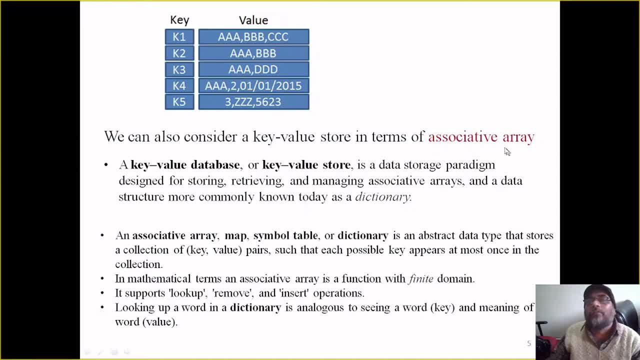 We can also consider key value stored in terms of associative array. If you understand the meaning of associative array in terms of mathematics, in terms of other kind of reasoning, Then everything will be easy To understand. Association array: you see here Some kind of association. it is. 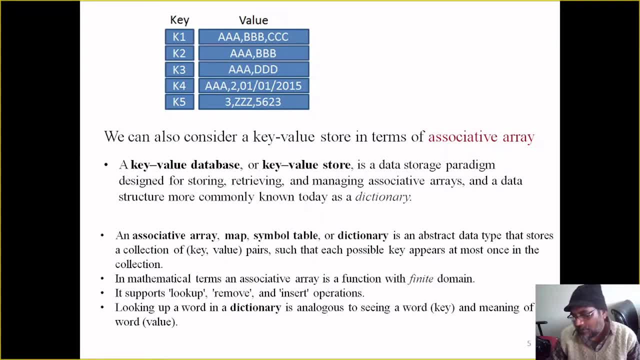 But we don't know what. So in some cases, when we formulate it by using some mathematical equation or formula, Then we say it is a simple function or a method. Okay, When association is some part. you see, When we see word in a dictionary. 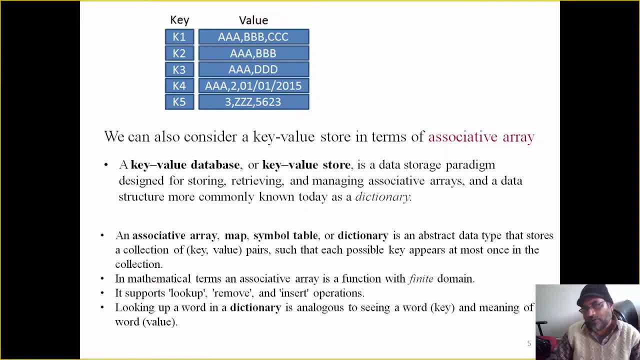 How do we search? Because the words in a dictionary they are arranged alphabetically, So we see a word alphabetically And wherever this word is present Along with we have its meaning and other details. That means the word that is unique in the dictionary. 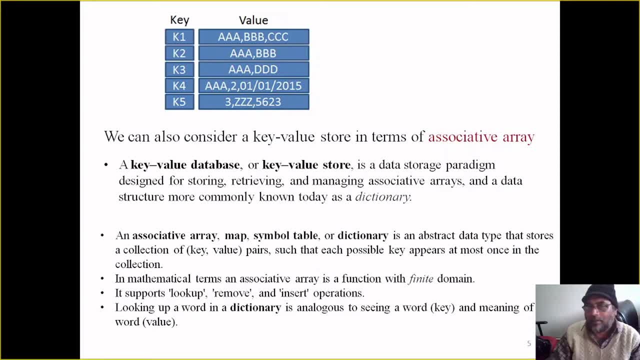 And is associated with this specific meaning. So this is a kind of association. Okay, So similarly, This key and value. When I say For this unique key value Or for this unique key, This is one specific data item, It is association with this one specific data item. 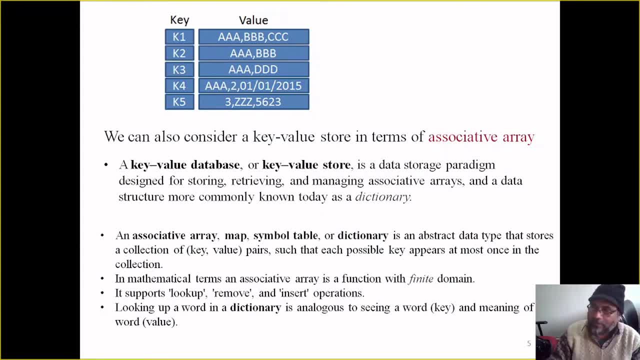 That means I am defining the association between key and data value Or data item, So it is a kind of association. And if I have this kind of association here So I can say it is a association or associative array, So we can consider, also consider the key value store in terms of associative array. 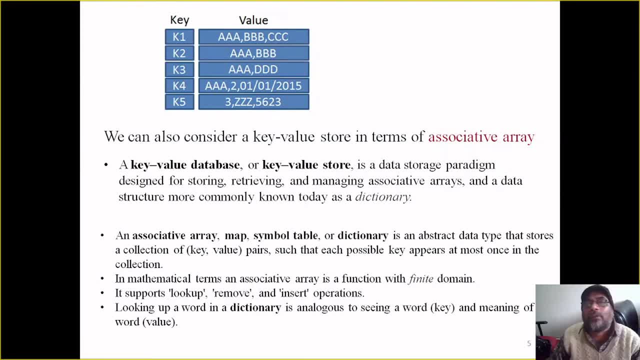 So key value database, or key value store, is a data storage paradigm Designed for storing, retrieving and managing associative arrays And a data structure More commonly known today as a dictionary. So you see, here It is just like if I say they are the words of dictionary. 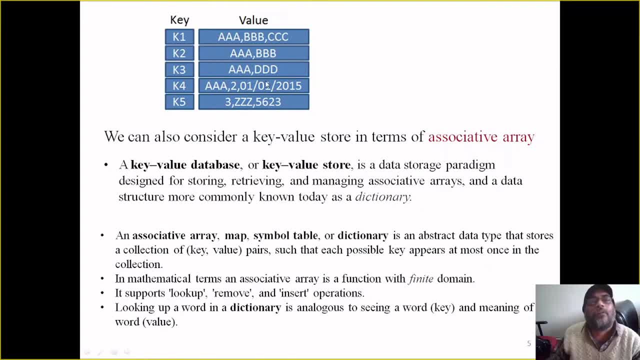 And it is the corresponding meaning of each word. Okay, So this kind of representation we call associative or associative array, So an associative array. We also have the different words Associative array, Map, Symbol, table Or dictionary Is an abstract data type. 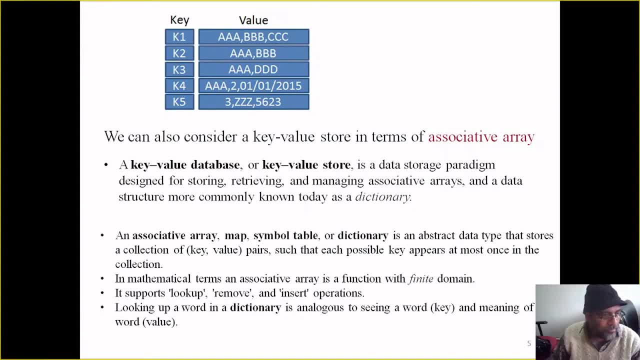 If we have some more higher level or some better mathematical reasoning, Then we say it is one abstract data type. That means I am saying it is a data type, But I am not talking about its actual implementation. It can have different form. So when I say abstract level, 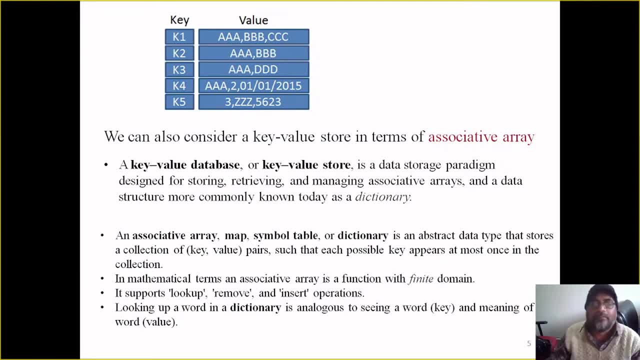 I am ignoring the details of implementation. So associative array, Maps, Symbol table Dictionary Is an abstract data type That stores a collection of key value pairs. Okay, You see here Key value pairs, Such that each possible key appears at most once in the collection. 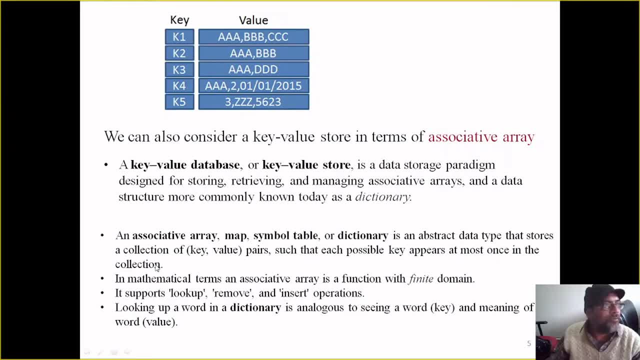 This should also Necessary because of it we have the uniqueness feature. In mathematical terms, an associative array is a function with finite domain. Okay, So it supports lookup, remove and insert operation. Now suppose this is our database, Then what kind of operations it should provide? 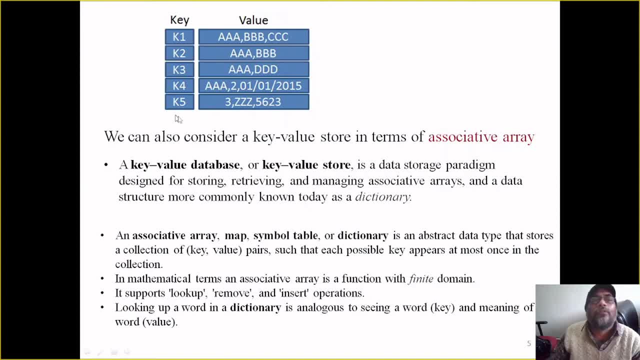 So generally what I can have, I can add one new key value item here, Okay. Second, I can remove any one of the key value item, Okay. Third, if I want to retrieve value for one specific key, Then I can have get kind operation. 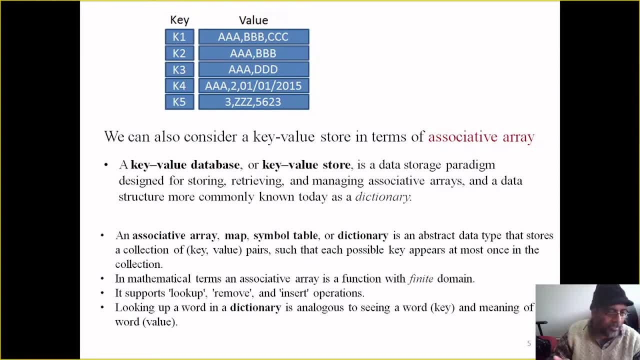 And here you will observe that only three kind of operations are proposed by the system. So lookup, remove and insert. So lookup is just like get, remove, delete and insert put Okay, So they may have some different name, But all have the same sense. 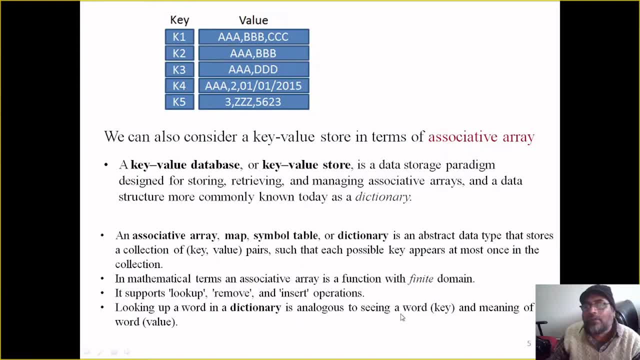 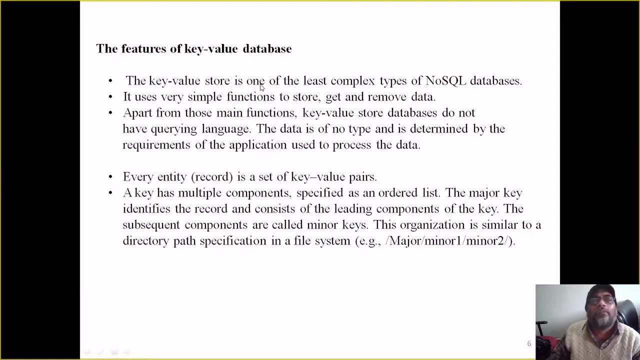 Looking up a word in a dictionary is analogous to seeing a word. So word means key and meaning of the word. that is the value. So some features are written here. The key value store is one of the least complex type of NoSQL database. 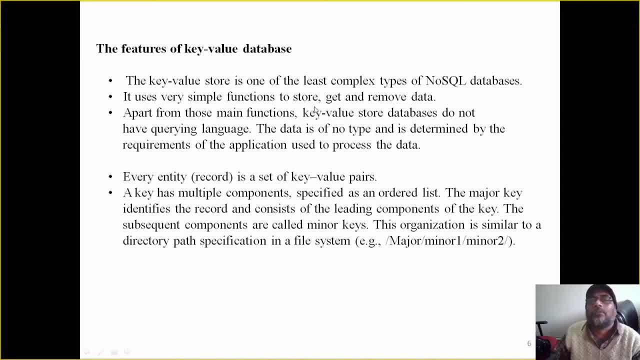 It uses very simple functions to store: Functions to store, to get and to remove data. Apart from those main functions- key value, store, database- do not have querying language. The data is of no type. The type definition is not here. No type And is determined by the requirement of the application used to process the data. 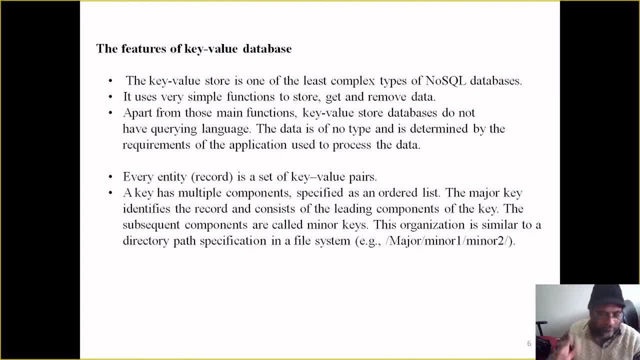 Application program written by the user of program. That will decide what kind format it is, What kind of this data is. Every entity or record is a set of key value pair. Okay, The records in the database will be only key value. key value, key value. 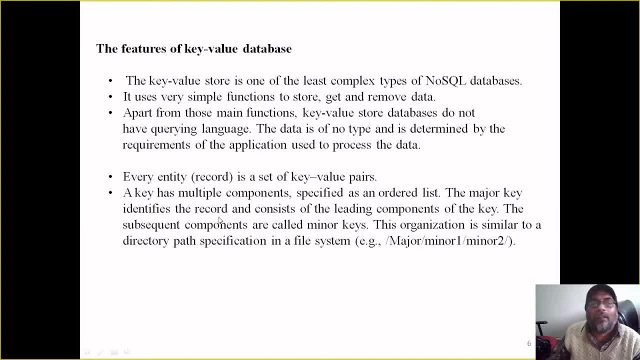 The major key identifies the record and consists of leading components of the key You will find here. generally we have key in relational database integer type, some value. Here you will see key can be of larger size And key can have components. One can be major key, other can be minus key. 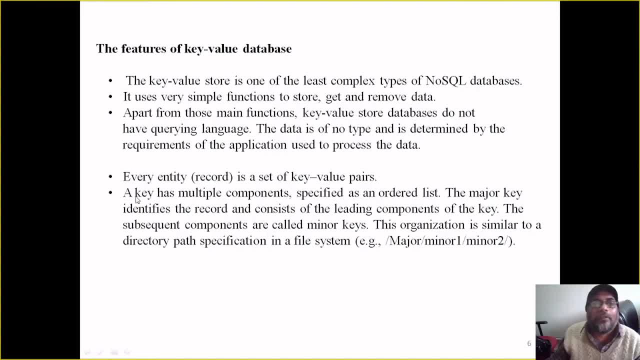 One part, other part, So the major key. The key has multiple components. It is specified as an ordered list. The major key identifies the record and consists of the leading components of the key. The subsequent components are called minor keys. The organization is similar to a directory path specification in file system. 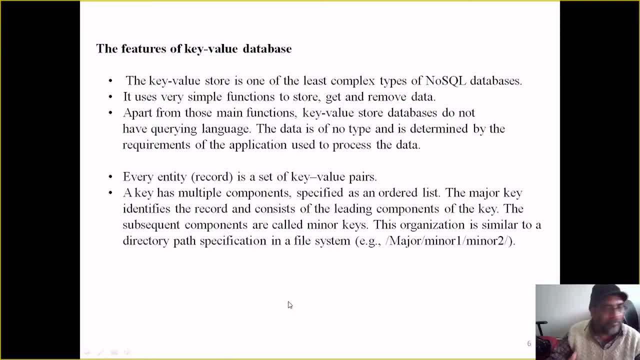 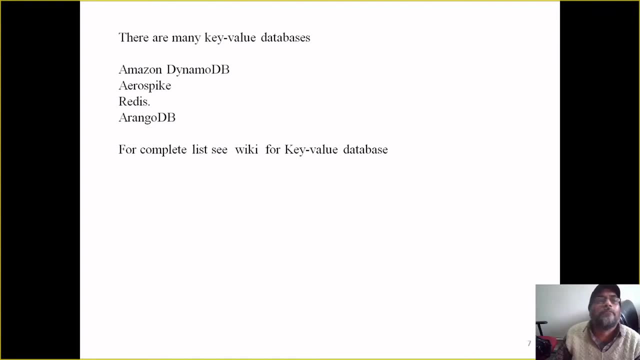 Generally in path and in operating system or file path Generally, we define this directory, then this subdirectory and finally this is a file. Same kind of notation is used here And there are many key value databases. Okay, And Amazon DynamoDB Arrow Spike. 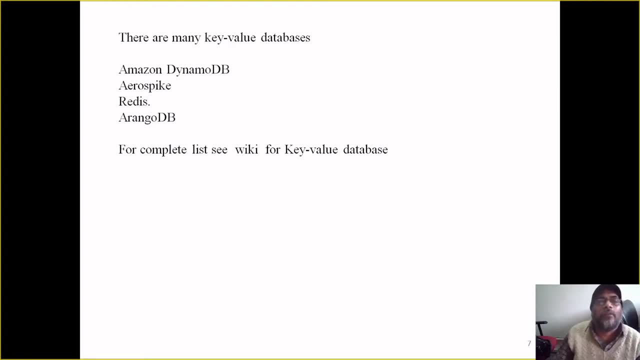 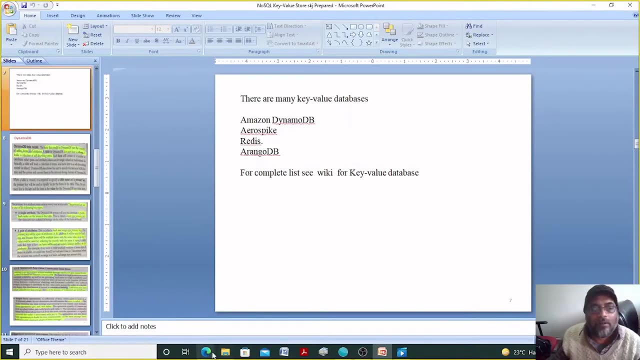 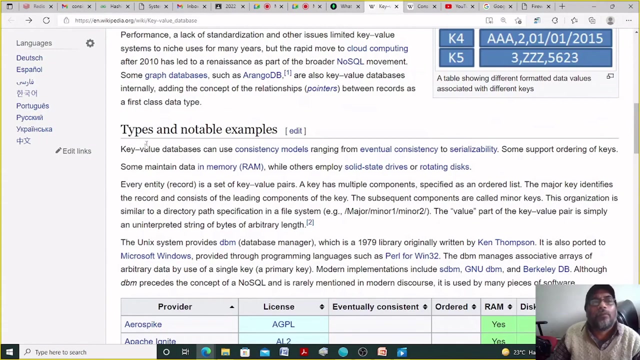 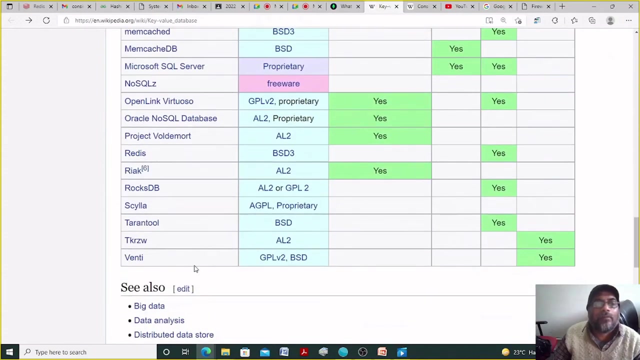 Redis, ArangoDB And complete list. I will show you on Wikipedia Where you will find the whole list. Okay, Here, this is key value database You can also see here. This is one. This is list of key value data store. 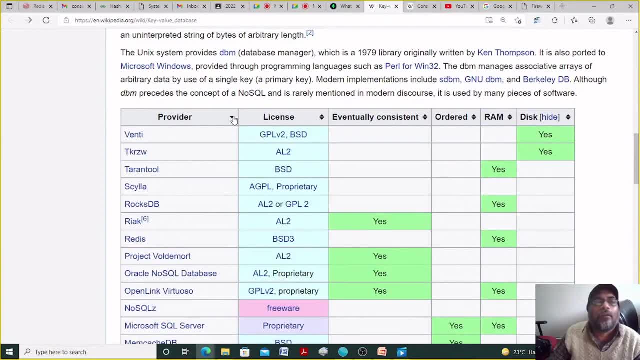 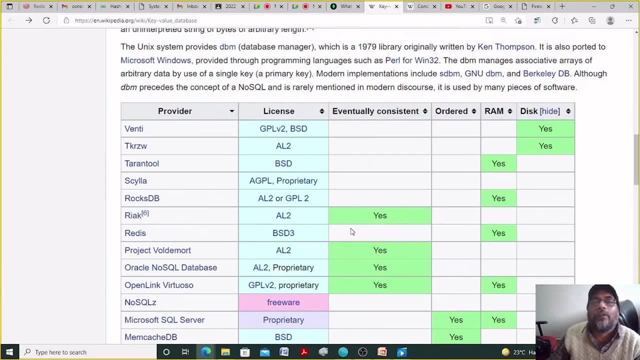 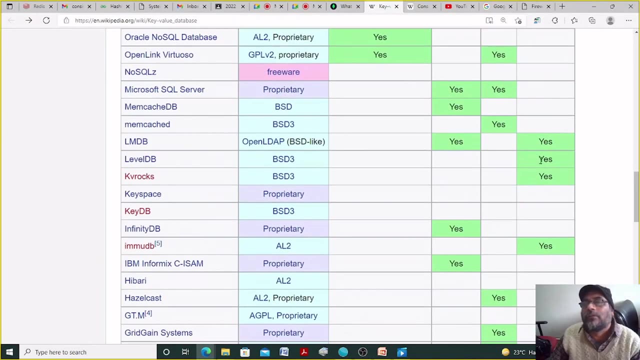 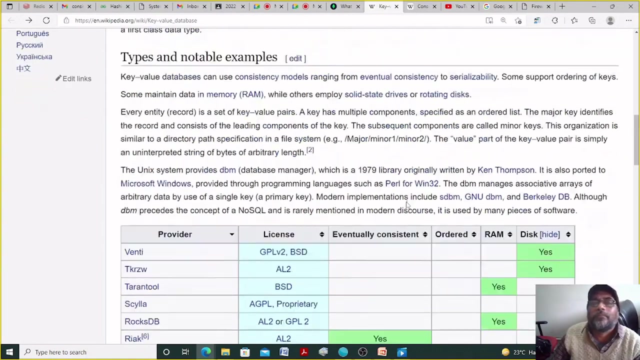 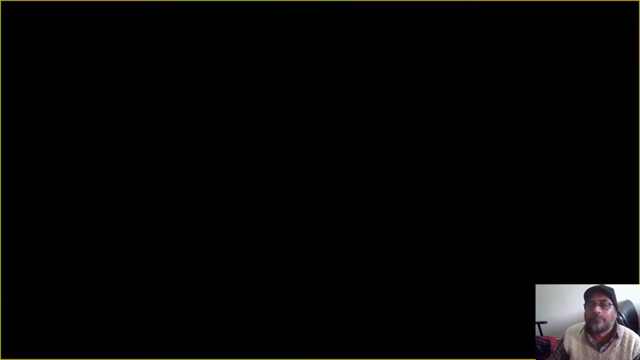 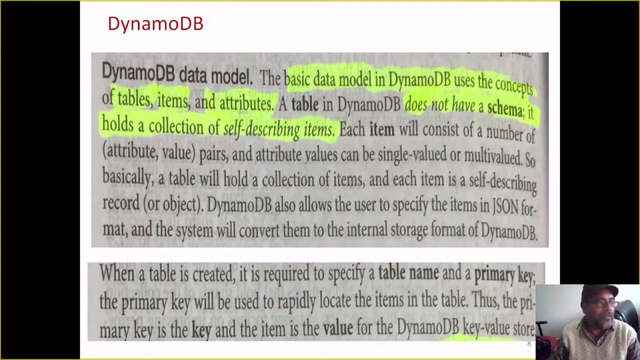 Here you see provider, license: open source or BSD or proprietary- Okay, Eventual consistency Program or disk where it is stored. Okay, So now I go back, So we will discuss this dynamoDB, This key value data store. 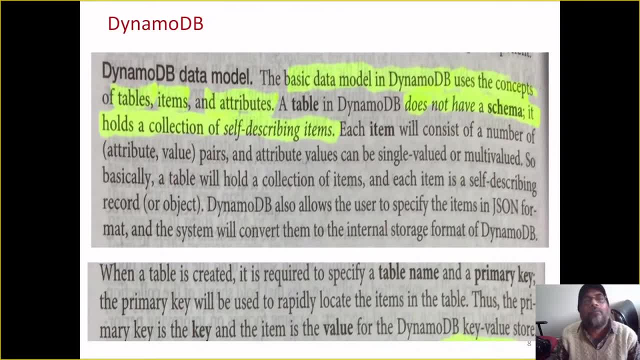 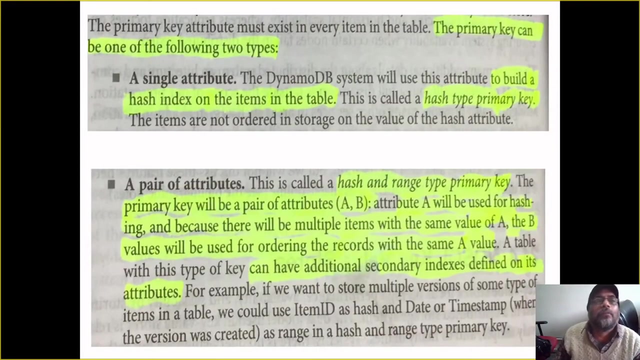 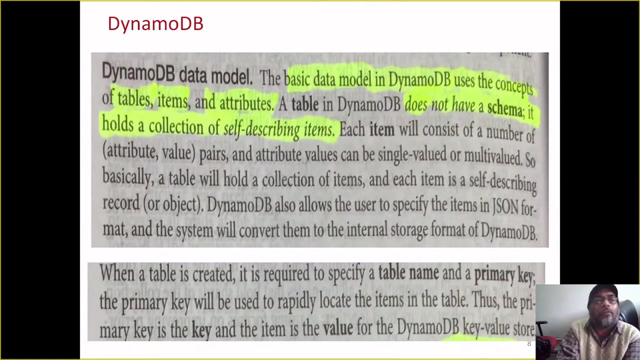 and you will try to understand how it does work. DynamoDB data model. the basic data model in DynamoDB uses the concept of tables, items and attributes. This is DynamoDB. it is a key value data store and it is amazing product. A table in DynamoDB does not have a schema. it holds a collection of self-describing items. 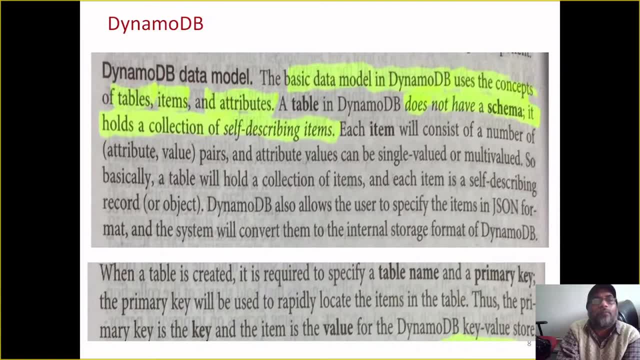 Each item will consist of number of attribute value pairs. The attribute value is the number of items in the table. Value can be single-valued or multi-valued. So basically, a table will hold a collection of items and each item is self-describing record or object. 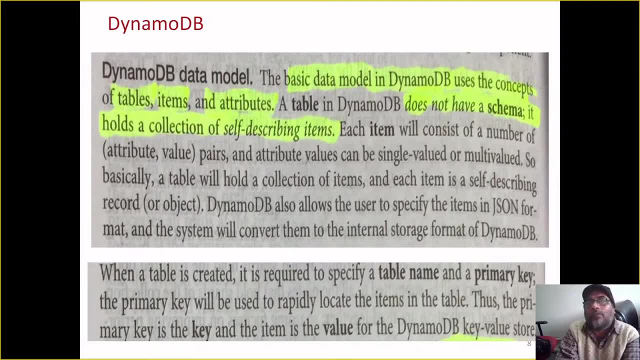 DynamoDB also allows the user to specify the items in JSON format and the system will convert them to the internal storage format of DynamoDB. When a table is created, it is a product of Amazon. When a table is created, it is required to specify table name and primary key. 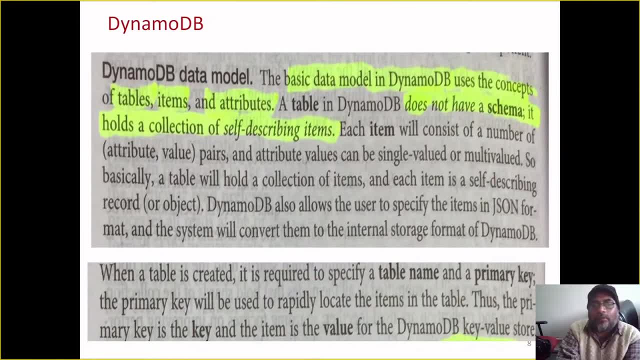 The primary key will be used to rapidly locate the items in the table. Thus, primary key is the key and the item is the value of DynamoDB key value store. This is the DynamoDB. it is a Amazon product and is available as part of Amazon web service or software development kit. 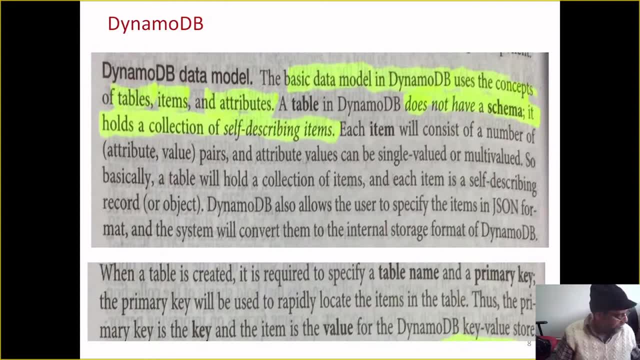 Thank you for watching this video. Amazon- It can be used as part of Amazon cloud computing services for data storage component. So Amazon, it is a product of Amazon and it is proprietary. also, We will see in next slide. The primary key attribute must exist in every item in the table. 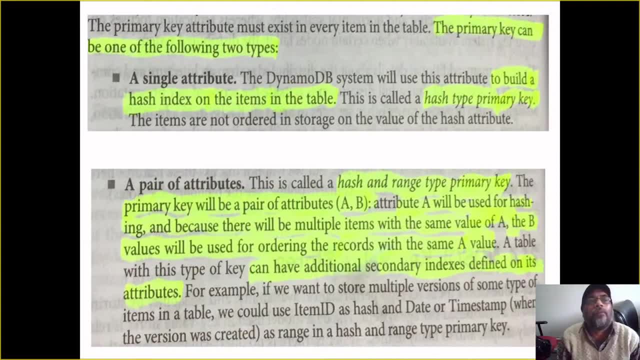 The primary key can be one of the following two types: Single attribute: The DynamoDB system will use the attribute to build a hash index on the items in the table. This is called hash type primary key. The items are not ordered in the storage on the value of the hash attribute. 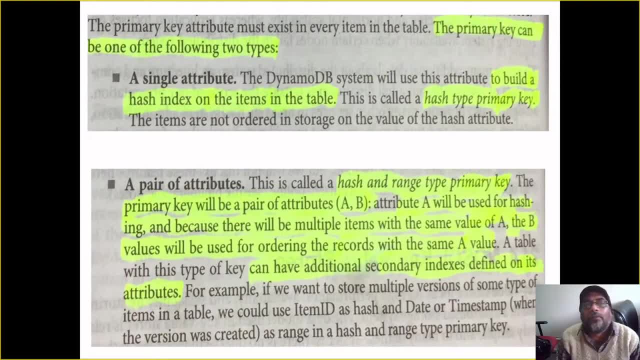 Pair of attributes. Pair of attributes. This is called hash and range type primary key. The primary key will be a pair of attributes: A and B. Attribute A will be used for hashing Hashing and, because there will be multiple items with the same value of A, The B values will be used for hash and range type primary key. 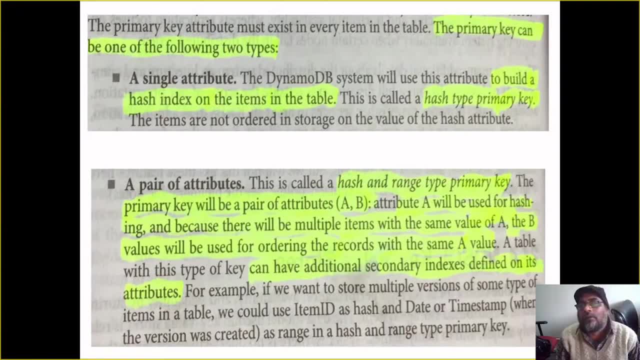 The B values will be used for hash and range type primary key. The B values will be used for hash and range type primary key. And the B values will be used for hash and range type primary key. The B values will be used for ordering the records with the same name A value. 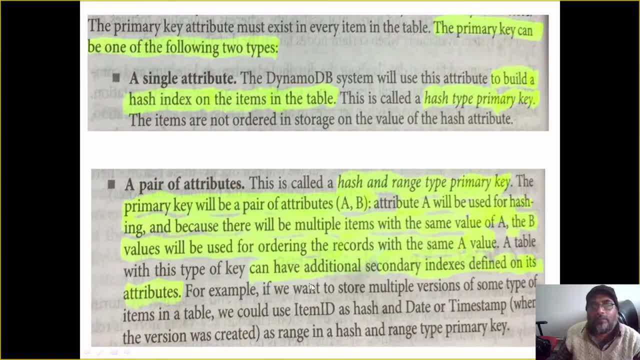 A table with this type of key can any additional secondary indexes defined on its attribute. For example, if we want to store multiple versions of the same type of items in a table, item id as hash and date on time stamp when the version was created as the as range in. 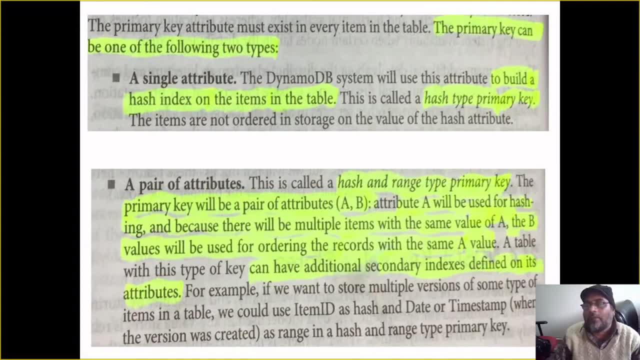 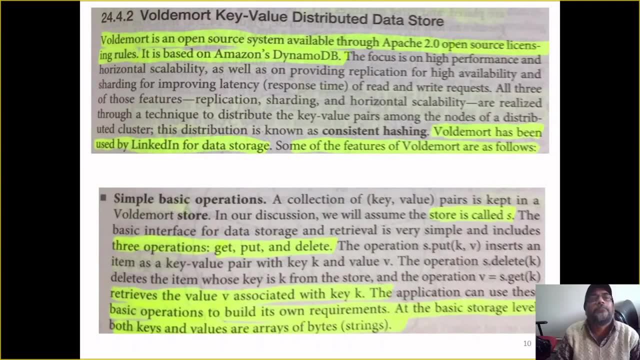 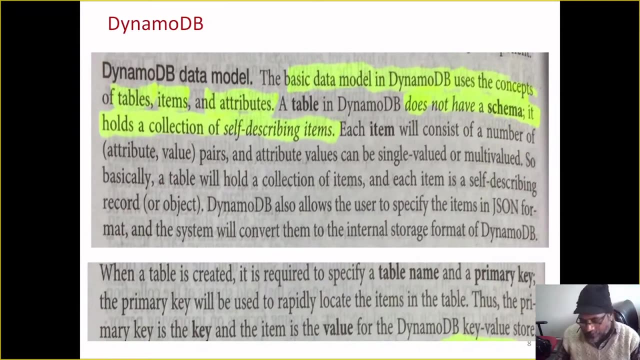 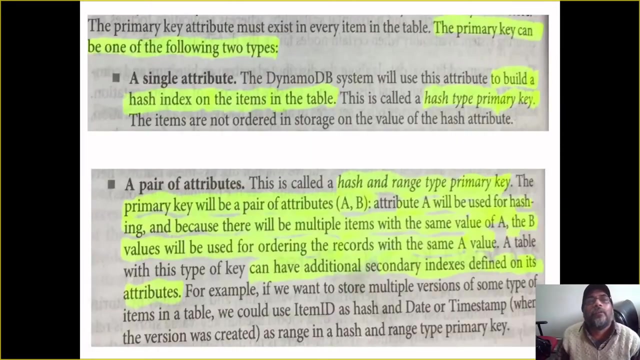 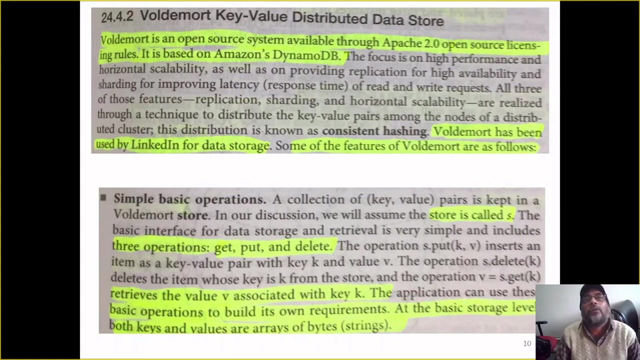 hash and range type memory key. actually, this dynamodb it is a proprietary product, so other details are not available. so to understand this dynamodb, there is corresponding one open source key value store. so to understand other details, we discuss now voldemort key value distributed data store. voldemort is an open source system available through apache 2.0. 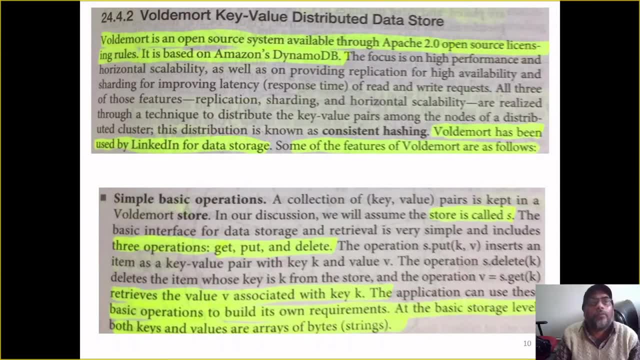 open source license licensing rule. it is based on amazon dynamodb. it has a similar kind of working as amazon dynamodb has the focus on high performance and horizontal scaling, as well as on providing replication of for high availability and sharding and for improving latency of read and write. request all three of those features: replication, sharding. 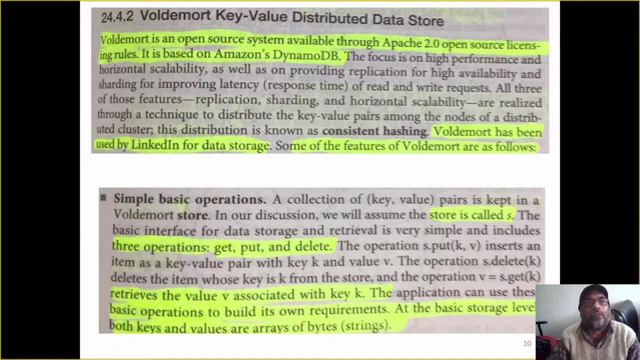 and horizontal scaling are realized through a technique to distribute key value pairs among nodes of our distributed cluster. the distribution is known as consistent hashing. i know this, what i was, I want to, I wanted to. so this consistent hashing, we will discuss. it is useful, okay. so distribution is known as consistent hashing. world remote has. 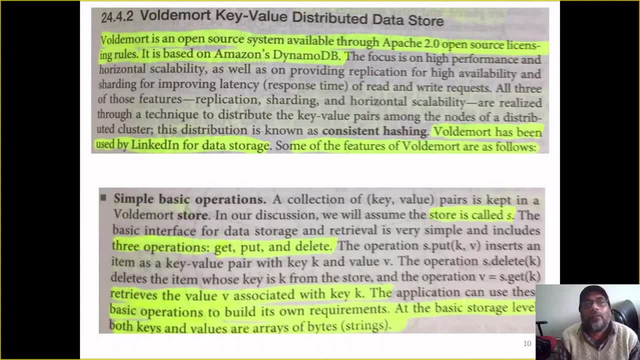 been used by linked in for data storage. some of the features of world world a mort are as follows: simple basic operation. a collection of key value pairs is kept in a world remote store. in our discussion we will assume the store is called X. okay, the basic interface for data storage and retrieval is very 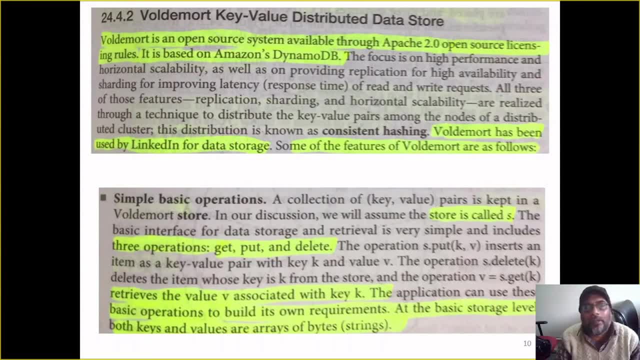 simple and include three operations: get, put and delete. the operation s dot put KB. this operation inserts an item in the key value pair with key K and value B. the operation s dot delete K deletes the item whose key is K from the store and the operation V, equal to s dot get K. 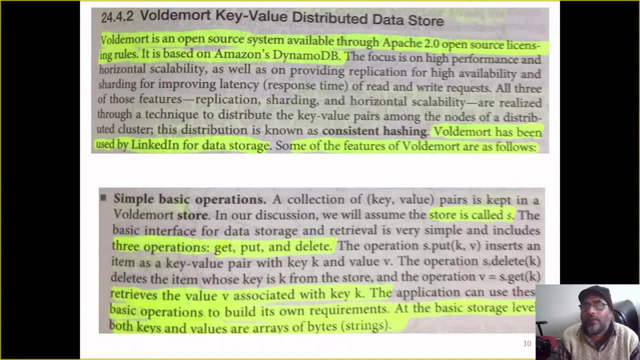 isout operand. safe is out. have information from the user pack. hold on full. has some crazy Python. there is another application called the Viking beat. there is a. it retreives the value we associated with the key K application. use these basic operation to build its own requirement. 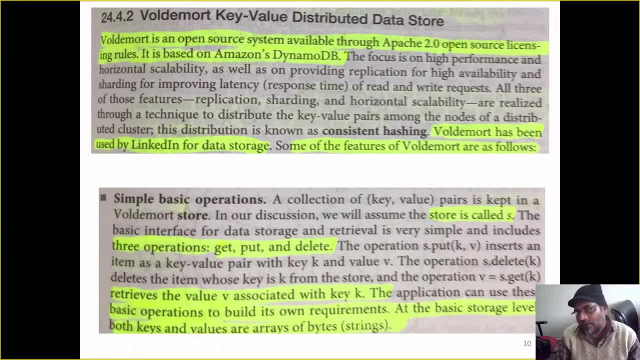 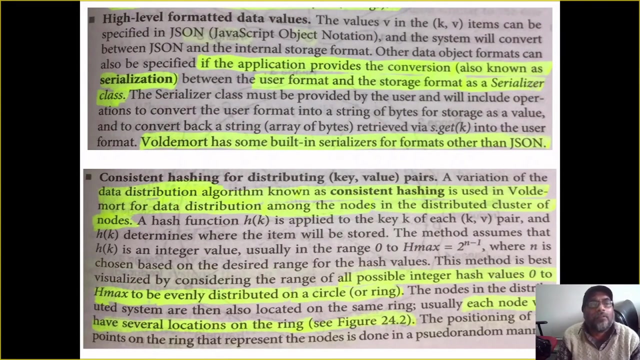 So using the combination of these one can decide a plan. So at the basic storage level, both key and values are arrays of bytes or strings. Second property: high level formatted data values and consistent hashing. for distributing So high level formatted data values, the values v in kv items can be specified in json javascript. 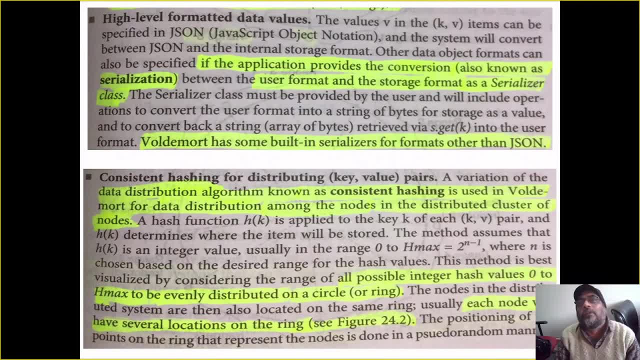 object notation and system will convert between json and the internal storage format. Other data object formats can also be specified. If the application provides high level formatted data values, the system will convert between json and the internal storage format. Third property provides the conversion, also known as serialization, between user format. 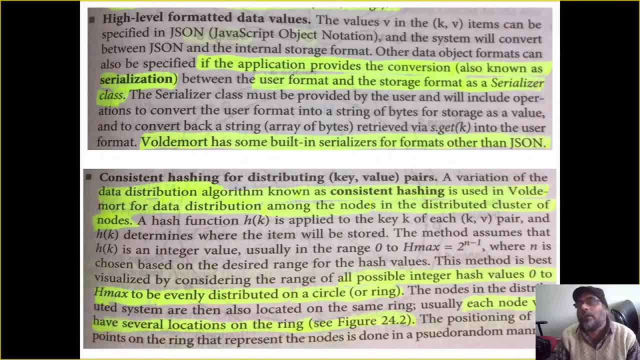 and storage format as a serializer class, So this is also present. The serializer class must be provided by the user and will include operations to convert the user format into string of bytes For storage array value and to convert back string array of bytes relative via get k into. 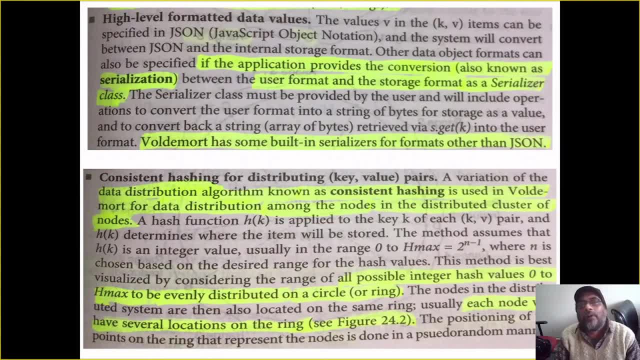 the user format. Valdemort has some built-in serializer for formats other than json, So other kind of formats can also be allowed here. So the serializer class can also be provided. The serializer is provided by the system. It takes care of converting the format. 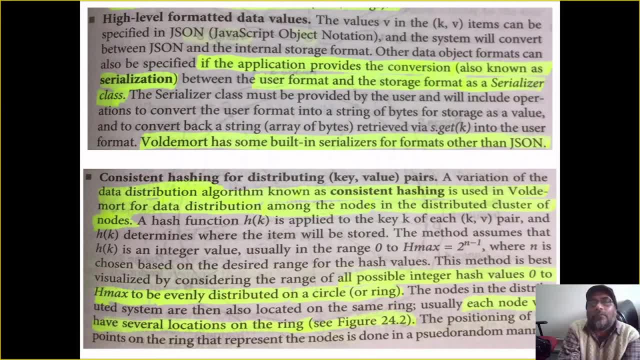 Then we have consistent hashing for distributing key value pairs. A variation of the data distribution algorithm known as consistent hashing is used in Valdemort for data distribution. Among the data distribution algorithm known as consistent hashing is used in Valdemort for data distribution. 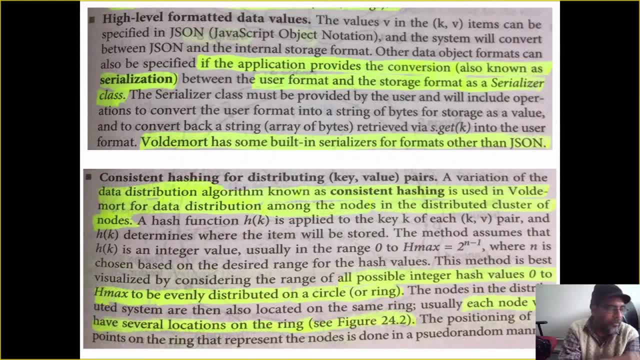 It is used in the distributed cluster of nodes. We will see here this consistent hashing is used at several places And what it is you will here see. all of you might be knowing the hash function. So in hash function, what we have? we generate numbers, integers in one range. 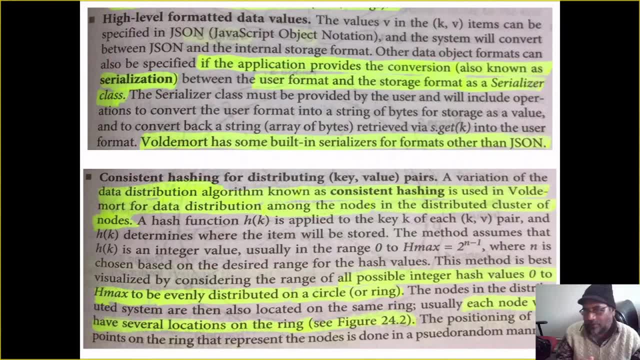 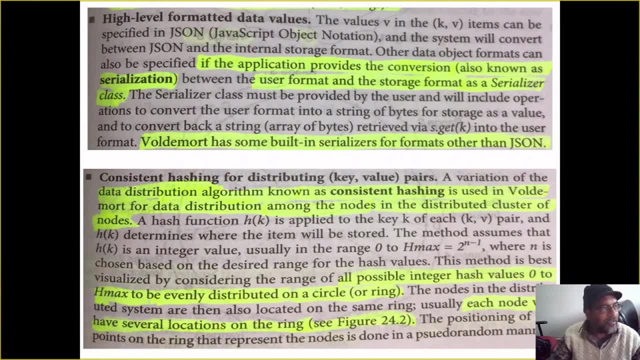 So that hash function can be used here, So that hash function needs some more, more folds, Not only here and in several other application. Not only here and in several other application. 1 example I can take. Suppose on cloud servicing there are several machine and on some machine load becomes. 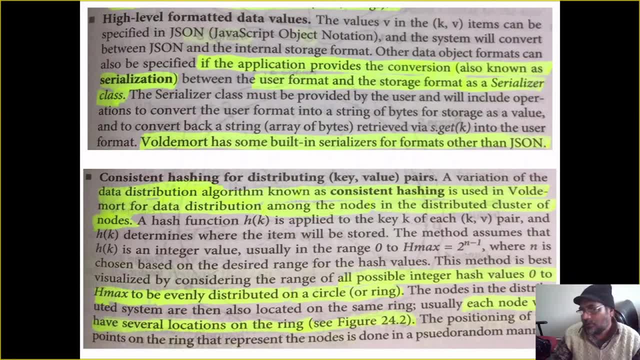 or some not machine. on some server load is more than the other And we want that this load may be distributed to the other server And we want that this load may be distributed to the other server. Who have 50,000 children to our service? 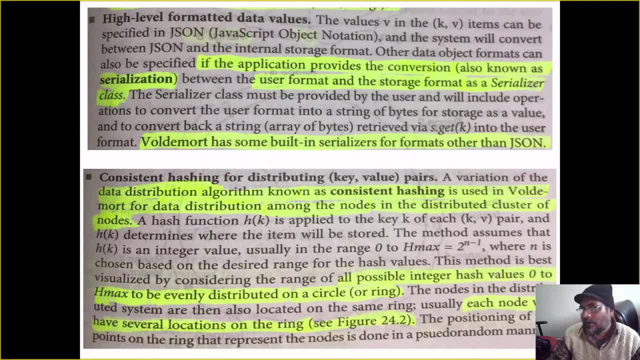 Who are having 27 or over individual kids, who has somewhat less load. so if we try to shift that load, what kind of exercise we have to do so that can be minimized by this hashing of consistent hashing. so consistent hashing can be used for distributed placement and it can be used for 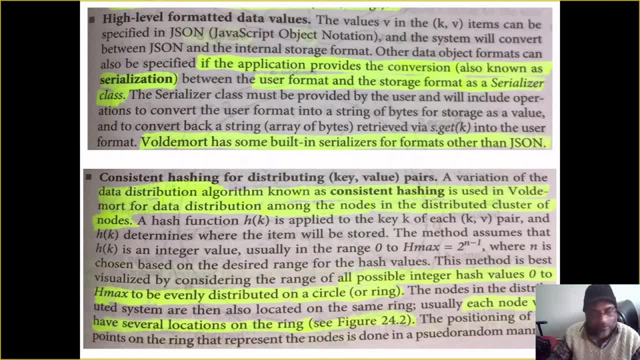 sharing load on in distributed or to manage sharing load in distributed environment so that overheads will be minimal. a variation of data distribution algorithm, known as consistent hashing, is used in Valdi mod for data distribution among the nodes in the distributed cluster of nodes. a hash function is applied to. 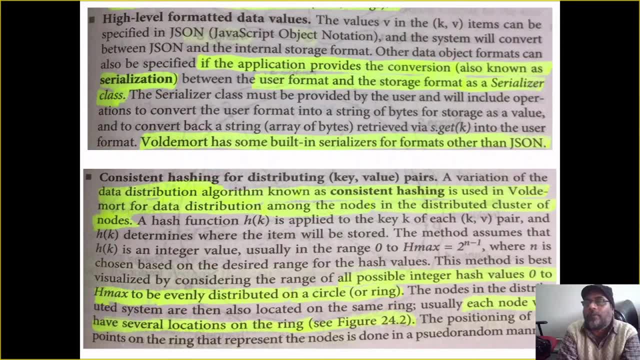 the key k for each kb pair, and hk determines where the item will be stored. the method assumes that hk is an integer value, usually in the range 0 to h, maximum to the power n-1, where n is chosen based on the desired range for the hash values. 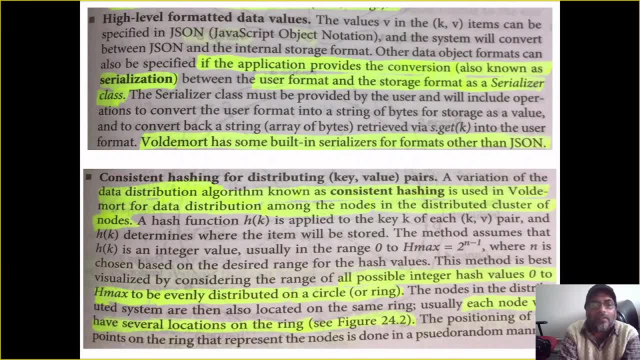 this method is best realized by considering the range of all possible integer has values 0 to h, maximum to be when evenly distributed on the circle or ring. the nodes in the distributed systems are then also located on the same ring. usually each node will have several locations on the same node. 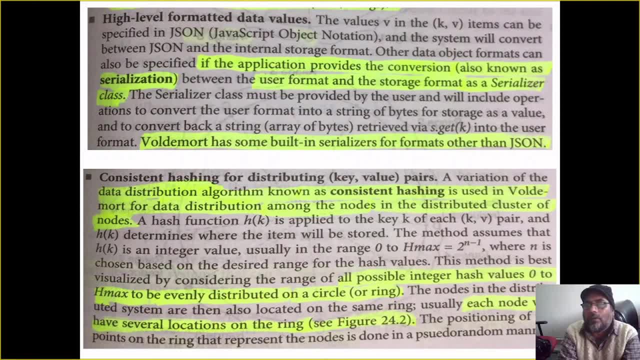 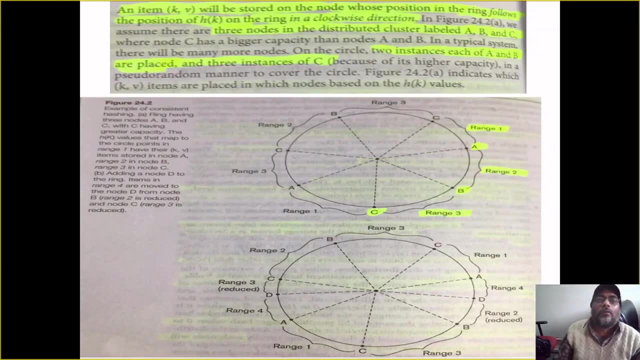 usually each node will have several locations on the same node. usually each node will have several locations on the same node, the ring. the positioning of the points on the ring that represent the nodes is done in a pseudo, random manner. so this diagram we have to discuss, you see here, suppose this: 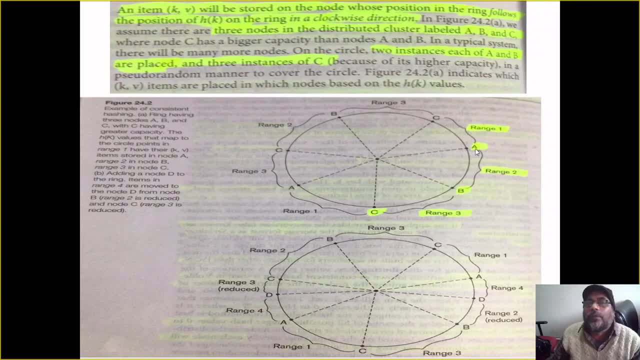 this is one circle and we have nodes A, B and C, we have key, value and item key and value. so suppose there are three nodes and we have several key and key have to be distributed on among these three nodes. ok, I want to keep so and so range of data on this node and that node, and